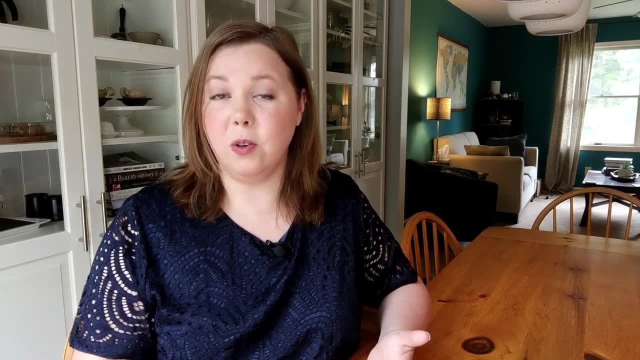 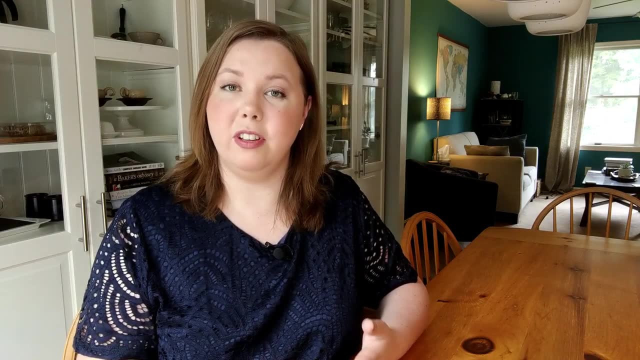 about analytical thinking in the last video. one of the things I mentioned was asking questions about how you could break down your problem into several smaller problems. This can help when you need to make assumptions too. Let's consider an analytical problem that you're likely to face. You're inviting 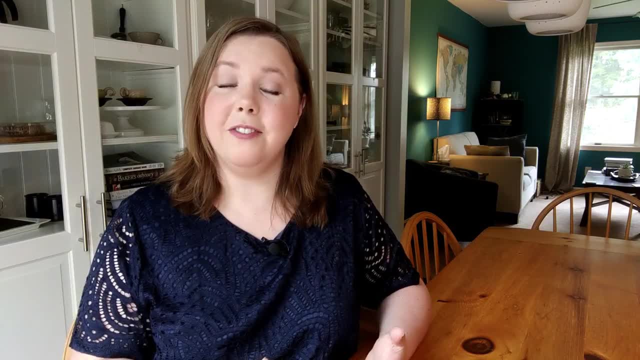 people over for a party and you're planning to serve dinner. You need to figure out how much food to get so that you have enough for everyone but that you don't have 10 times the amount of food that you need. Let's see how that. 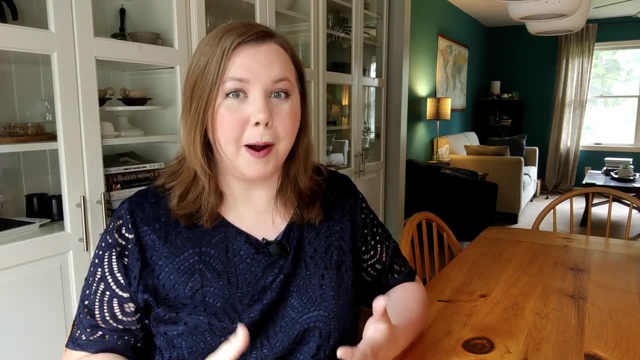 works for you. You know you need to raise an amount of food, but you have just 10 times the amount for anyone. And if the food was enough for everyone, it'sena. How do you solve this? The real problem is how much food will be eaten. 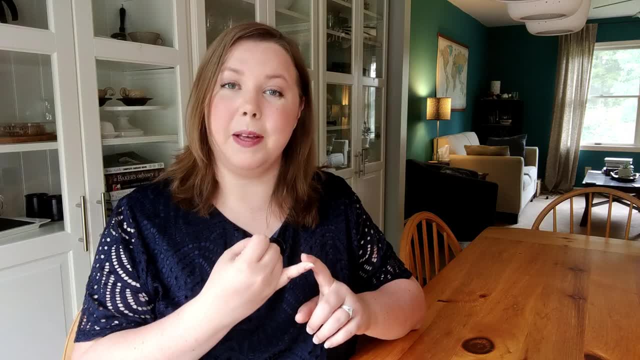 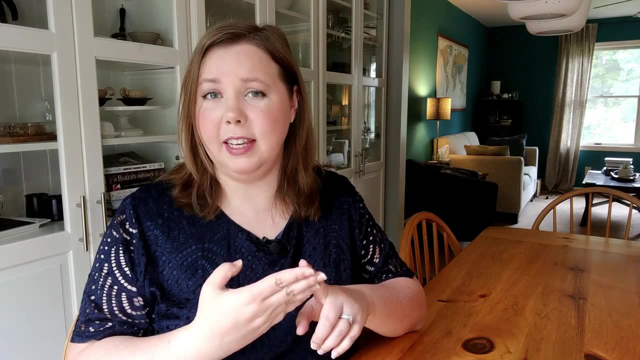 The pieces you can break this down into are: how many people am I inviting, How many people are likely to come, How many different items am I going to serve, And how much of each are people likely to eat? The answer to all of these are likely guesses, but you can make some educated assumptions. 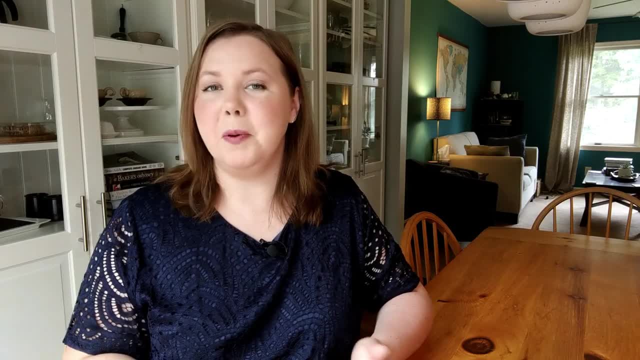 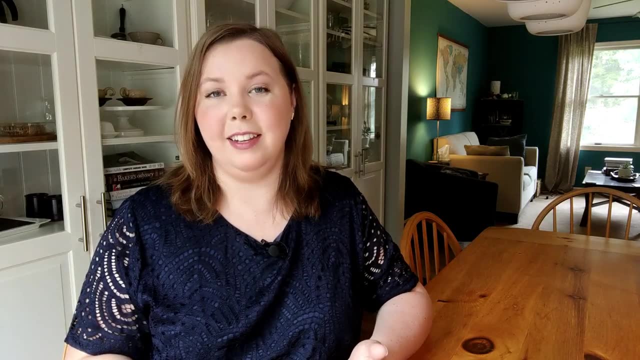 You'll figure out approximately how many people will show up. Some people will immediately say they can't come because they have other plans, And there may be other people that, while you invite them, you know they're unlikely to show up. You can estimate how much food people are going to eat. Having hamburgers and hot dogs. If it's mainly children, maybe you assume one hot dog or one hamburger per kid. Is the group mostly teenagers? Maybe count on a few of each. Have vegetarians coming, Count in a few veggie hot dogs or hamburgers. 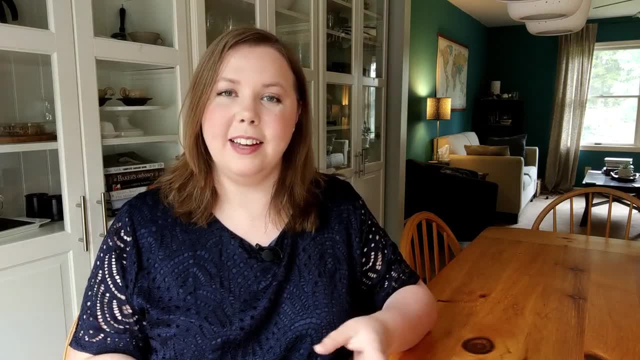 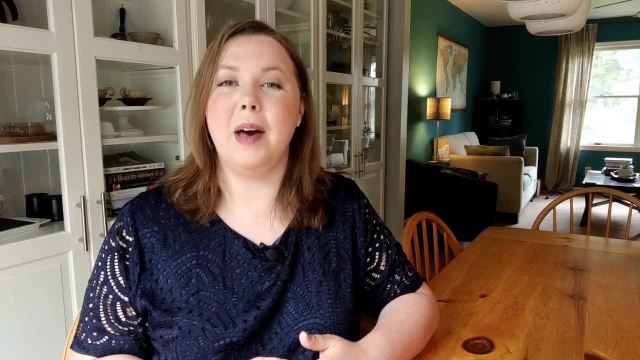 You can take the same approach with any problem: Break it down into pieces and then make the best assumptions you can. I always recommend making a note of your assumptions so that you can go back and see what assumptions you made if things went wrong or if you maybe need to adjust. 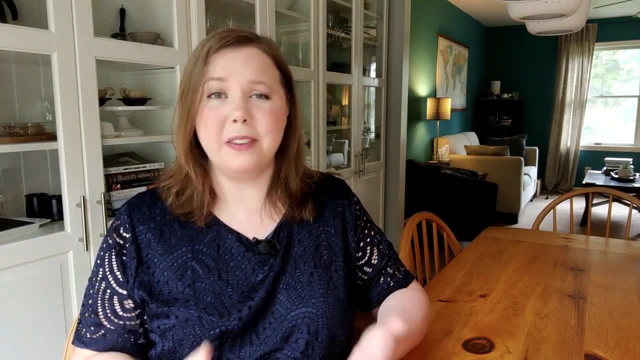 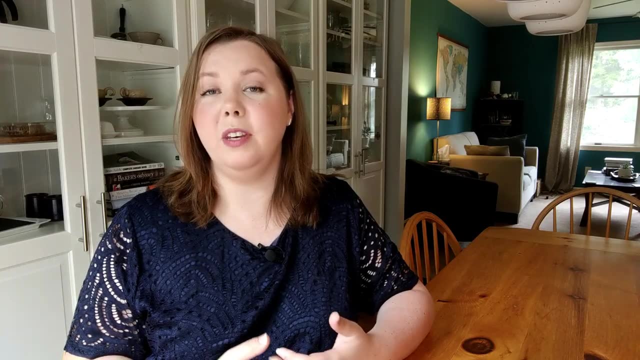 Let's talk more about creating actionable solutions. What's the best way to do this? Let's stick with the same example. Maybe you're getting something that's a more expensive ingredient, and so you need to know pretty precisely how many people are coming. 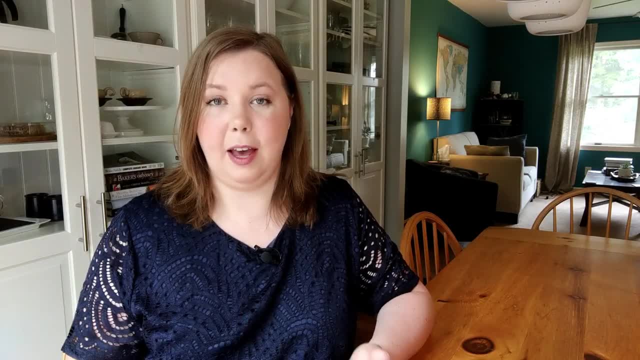 You could ask people to RSVP. This will tell you exactly how many people will be showing up when you come. You could ask people to RSVP. This will tell you exactly how many people will be showing up when you come. You could ask people to RSVP. 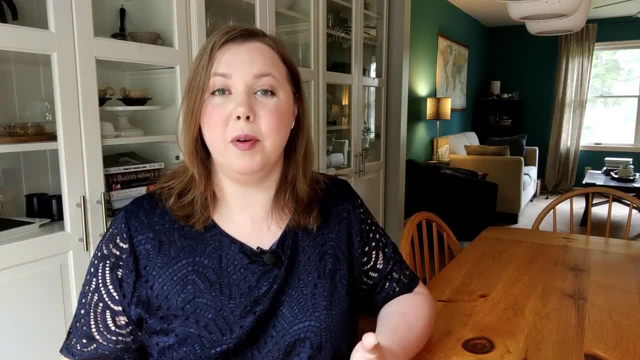 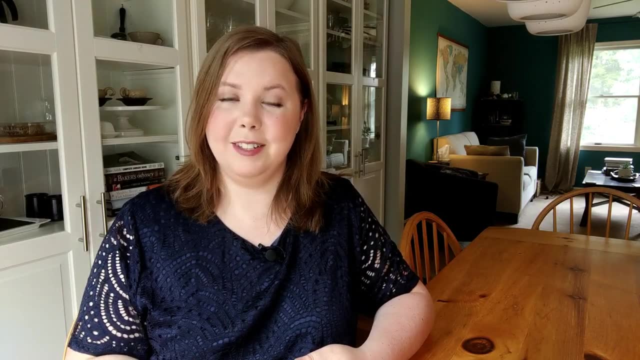 This will tell you exactly how many people will be showing up when you have that dinner. This eliminates one of your assumptions, which makes your number more concrete. You are probably already using more analytical thinking skills in your daily life than what you realize. Problems like the one I mentioned occur in thousands, if not more, households- every single.